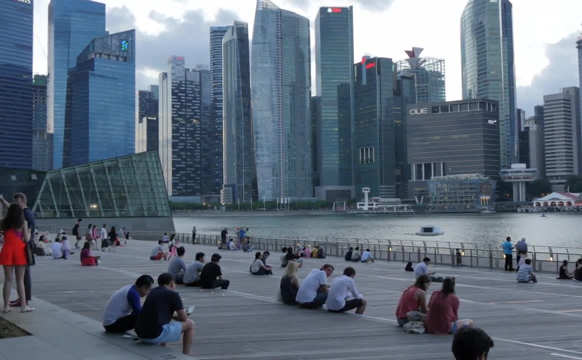 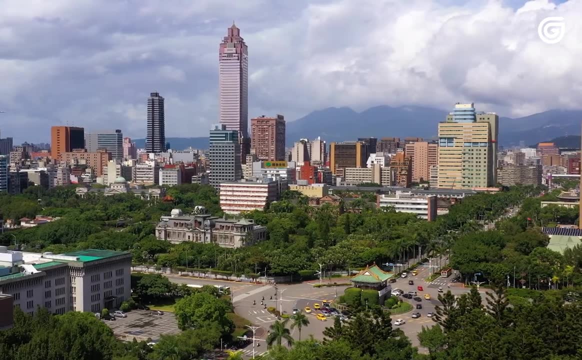 world History of the Asian Tigers is a story of determination, resilience and the transformative power of economic freedom and good governance. These countries serve as a valuable example for future generations of policymakers and business leaders who are seeking to drive economic growth and prosperity. 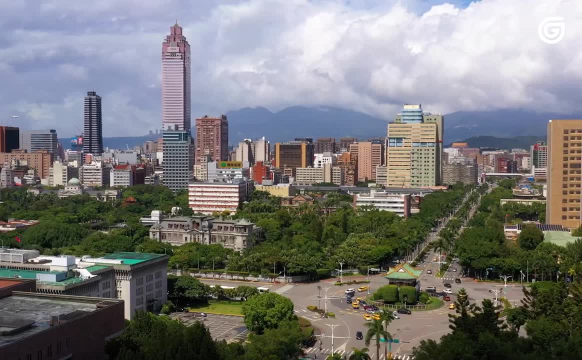 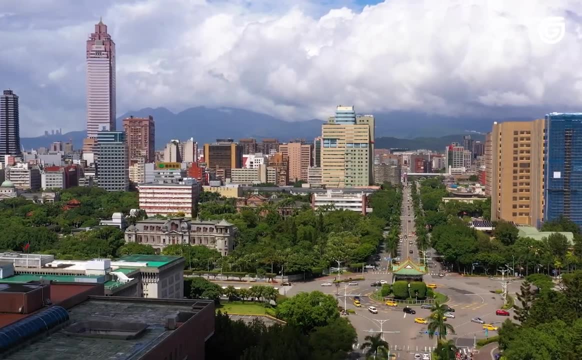 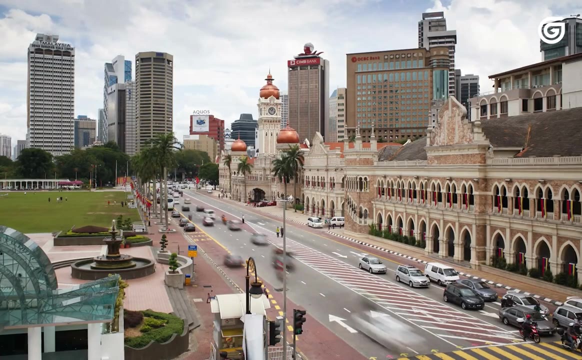 In addition to the original four Asian Tigers of Hong Kong, Singapore, South Korea and Taiwan, there are several other countries in Asia that are often considered to be part of the group. Some of these include Malaysia, Thailand and Indonesia. These countries share similar characteristics with the original Asian Tigers, such as high. 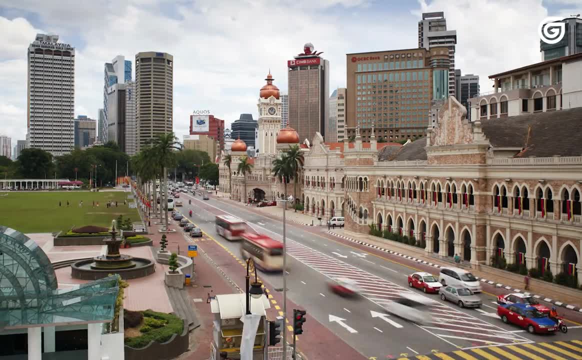 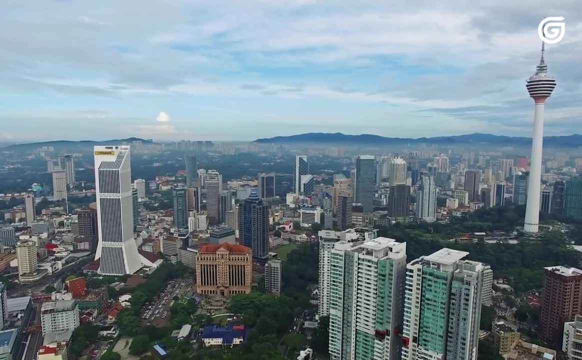 levels of economic growth, rapidly developing economies and a focus on export-oriented industries. They have also demonstrated an ability to compete. The Asian Tigers are seen as a major player in the international economy. Throughout Asia, there has been a growing recognition of the importance of economic 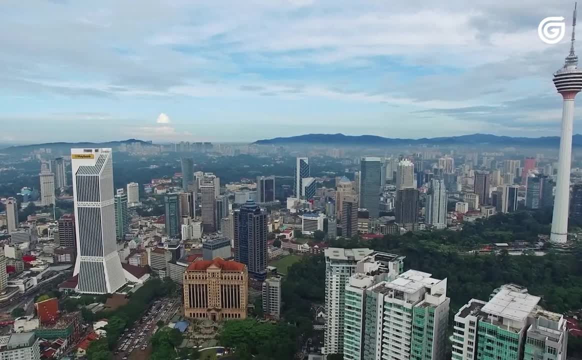 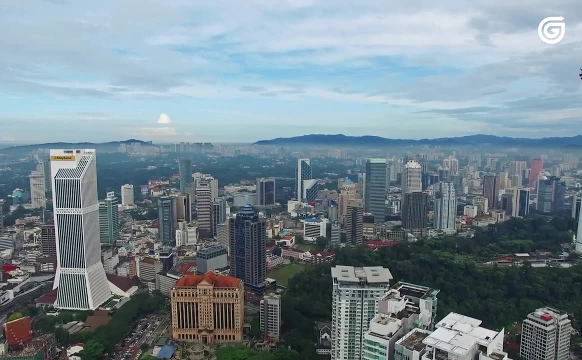 development, and many countries in the region have embraced economic reforms and liberalization to drive growth. This has led to the rise of several new Asian economic powerhouses, and the region as a whole has become a major player in the global economy. In recent years, Asia has been experiencing strong economic growth, driven by the rapid 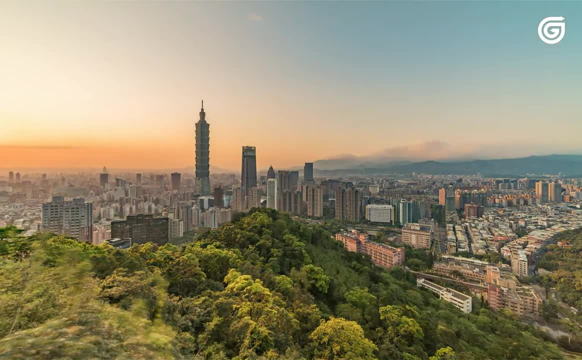 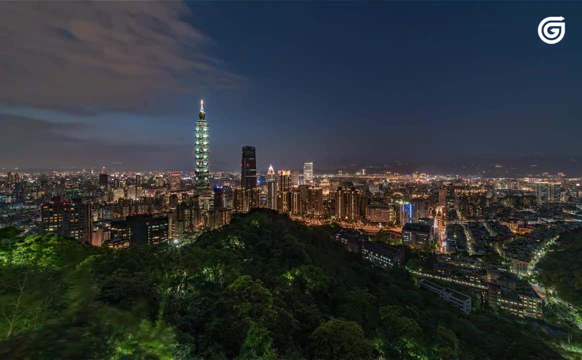 expansion of its manufacturing, technology and service sectors. The region is home to some of the most important Asian Tigers in the world. It is one of the world's largest and fastest-growing economies, and its growing middle class is increasingly becoming a major force in the global marketplace. 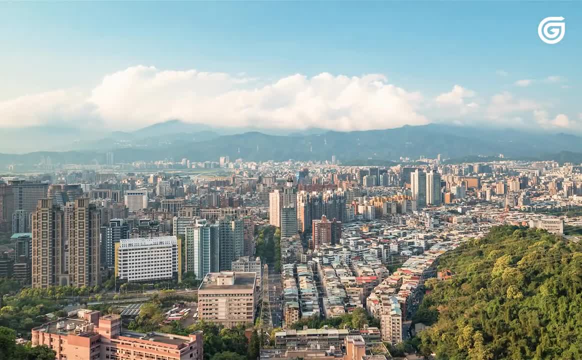 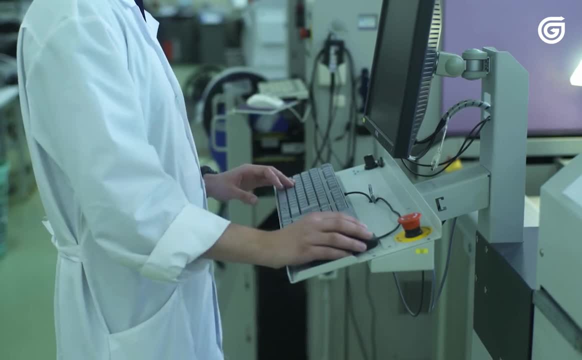 The Asian Tigers' economies boomed in a variety of industries, including manufacturing, technology and services. The development of strong, export-oriented manufacturing industries was a key factor in their success. For example, South Korea and Taiwan became leaders in the electronics sector, producing 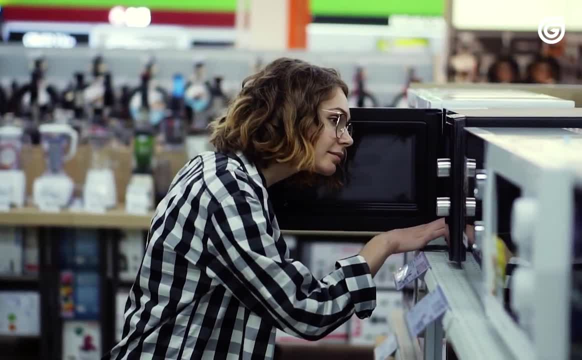 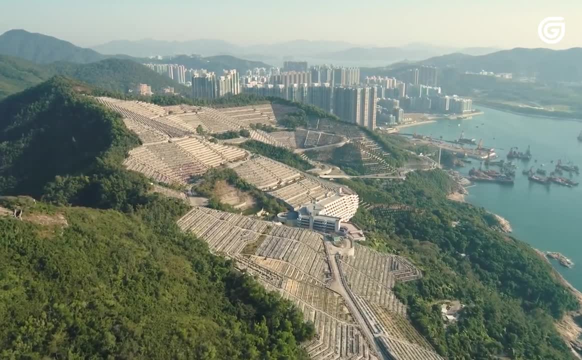 a wide range of products, such as televisions, computers and smartphones. Hong Kong and Singapore, on the other hand, have also been a major player in the global market. On the other hand, leverage their status as international trade and financial centers to drive economic growth. 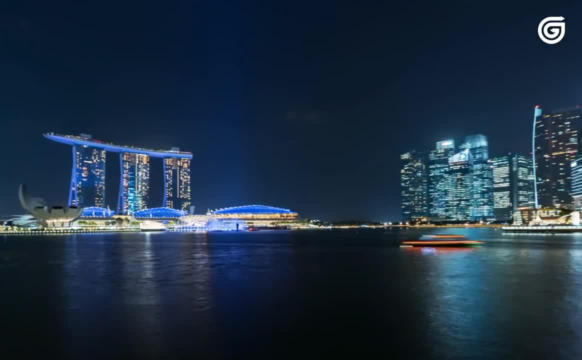 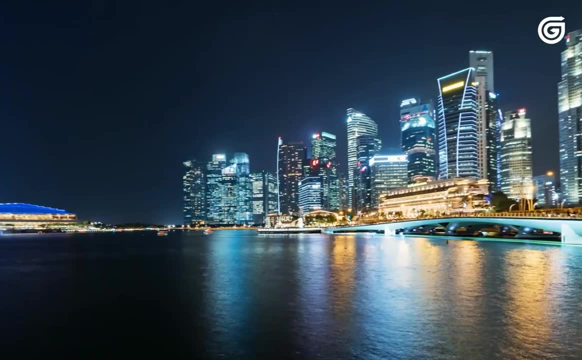 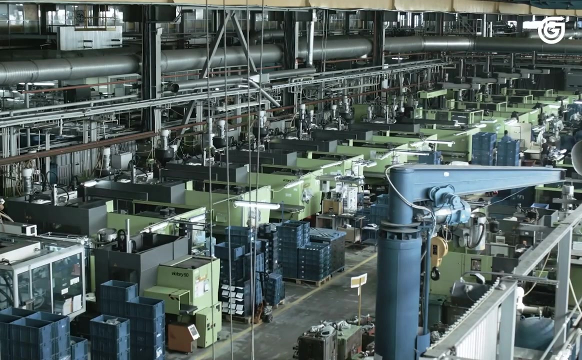 These countries developed sophisticated financial systems, a highly skilled workforce and supportive business environments that made them attractive to foreign investment and trade. In recent years, the Asian Tigers have continued to thrive, but they have also faced a number of challenges, For example, the manufacturing industry, which was once a key driver of their economic success.